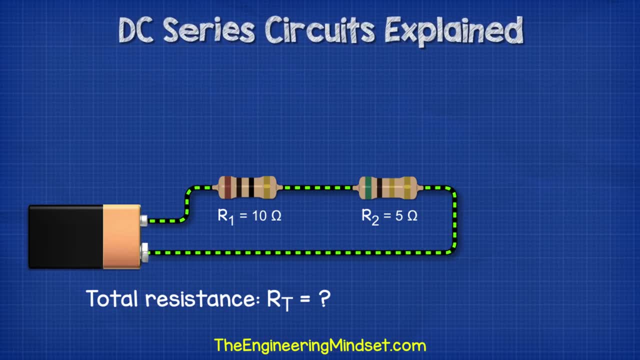 10 ohms. If we then added a second resistor- R2, with 5 ohms of resistance into the circuit, the total resistance is now 15 ohms. that's because 10 ohms plus 5 ohms. If we added another 5. 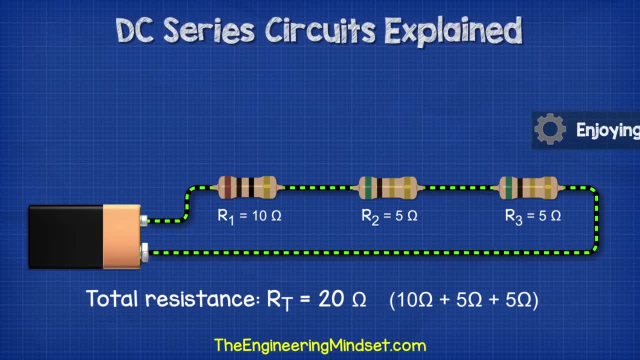 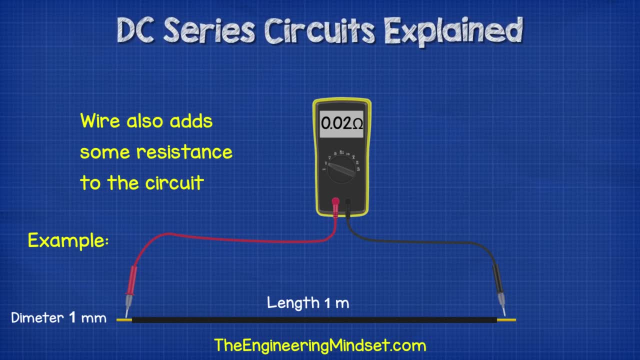 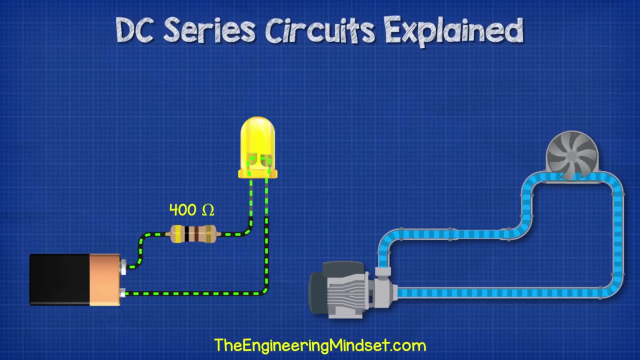 ohm resistor, then the total resistance is now 20 ohms. In reality, the wires too will add some resistance, but this is very small. You might need to account for this, depending on how accurate your design needs to be. Current in series: Current is the flow of electrons. It's like water which flows through. 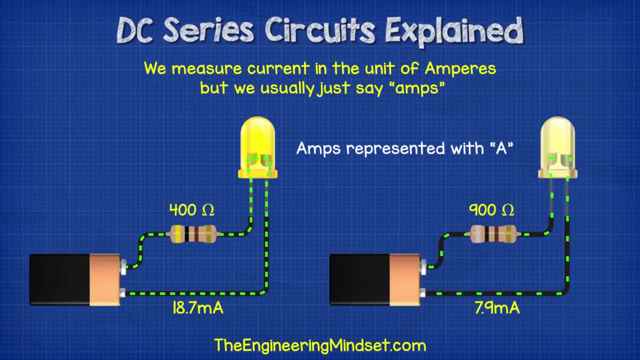 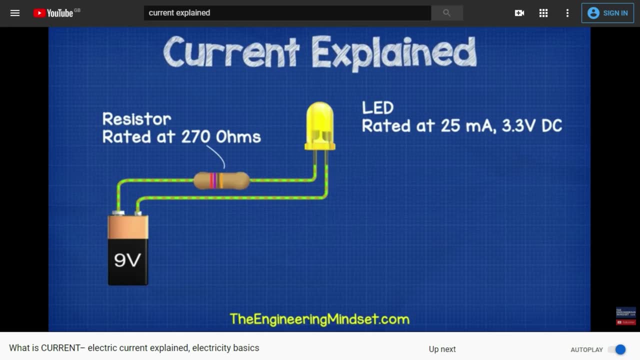 a pipe, The higher the current, the more electrons are flowing. We measure current in the unit of amperes, but engineers tend to shorten this to just amps. Now we have covered current in detail in our previous video. do check that out. links down below. 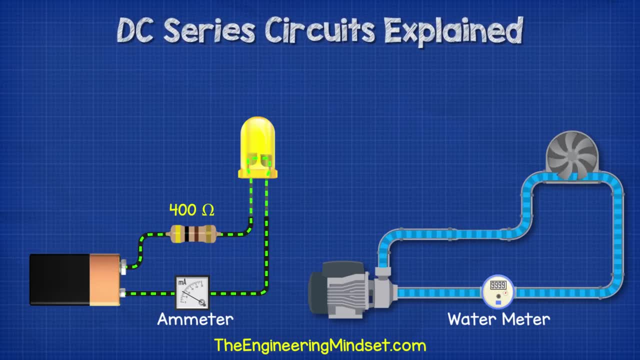 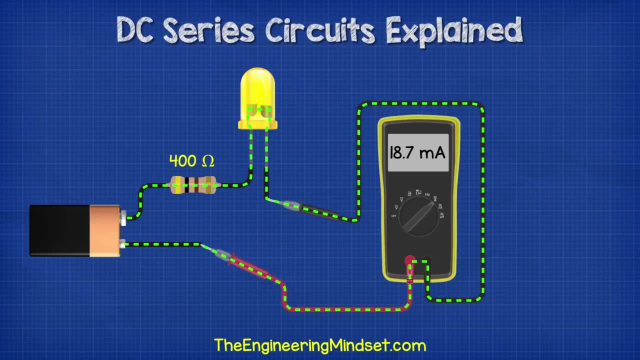 We measure current by placing an ammeter into the circuit for the electrons to flow through. This is like a water meter in the sense that water must pass through it for us to measure it. We can connect a multimeter into the circuit to also read the current. The multimeter must. 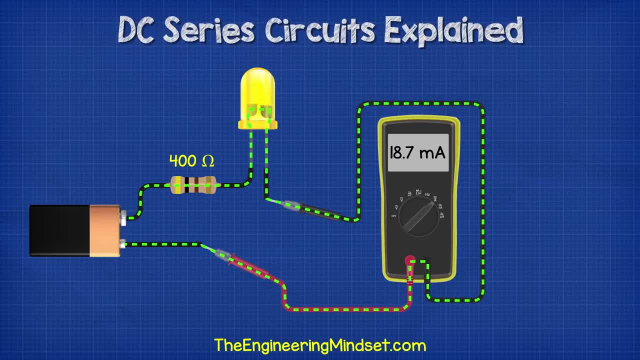 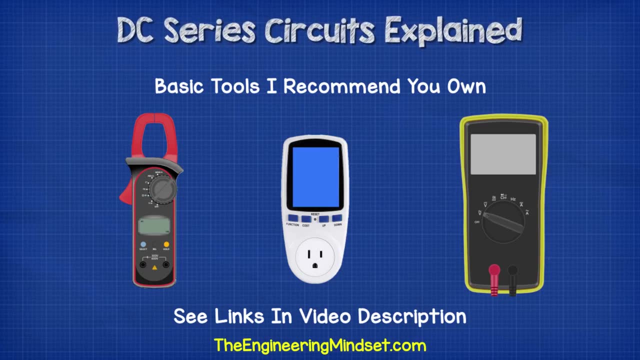 be placed into the circuit for us to take a reading, because the current is going to flow through this. The meter will add some resistance to the circuit, but it's such a small amount that we can usually just ignore this. If you don't have a multimeter yet, then I highly recommend. 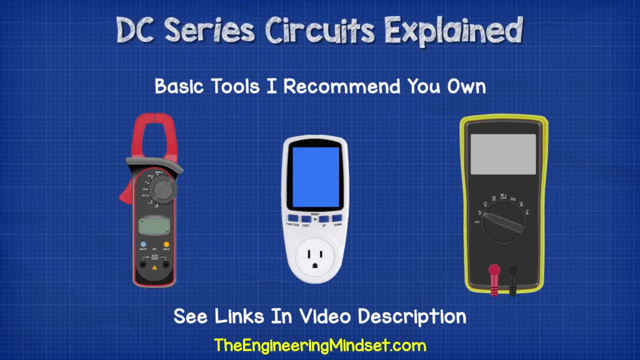 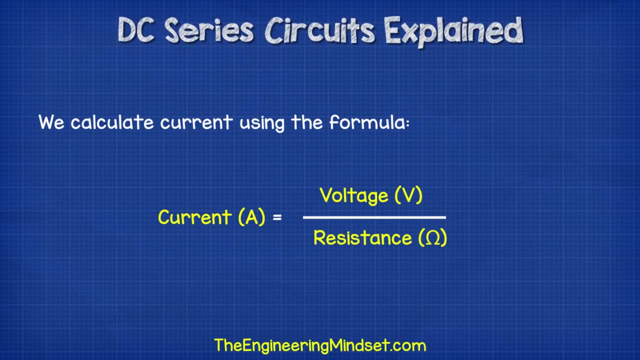 you get one. they are essential for troubleshooting and also building your understanding. I'll leave some links down below for which one to get and from where. We can calculate the total current of the circuit by dividing the voltage by the resistance. So if we connect a 10 ohm resistor to a 9 volt battery, 9 volts divided by 10 ohms gives 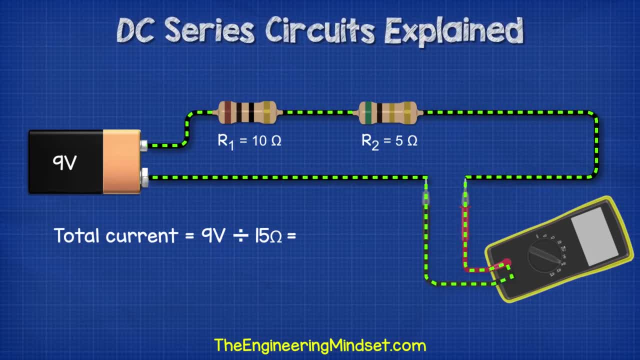 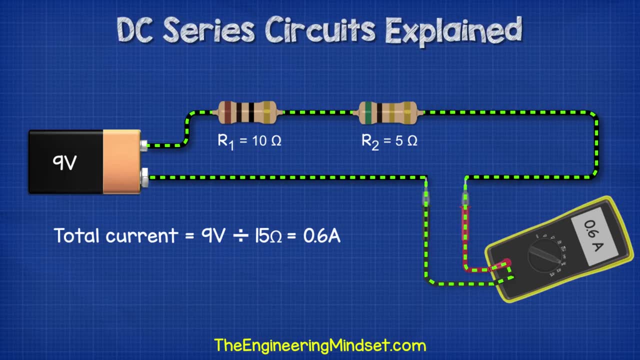 us 0.9 amps. If we added another 5 ohm resistor to the circuit, that gives us 15 ohms of resistance. so 9 volts divided by 15 ohms equals 0.6 amps. And if we added another 5 ohm resistor, that gives us 20 ohms of resistance, so 9 volts. 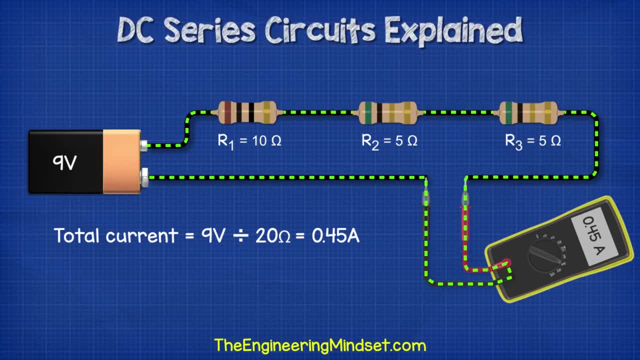 divided by 20 ohms equals 0.45 amps. So we can see that as we add more resistance to the circuit, the current reduces, so less electrons are flowing and that means we can do less work. We can visualise that by connecting. 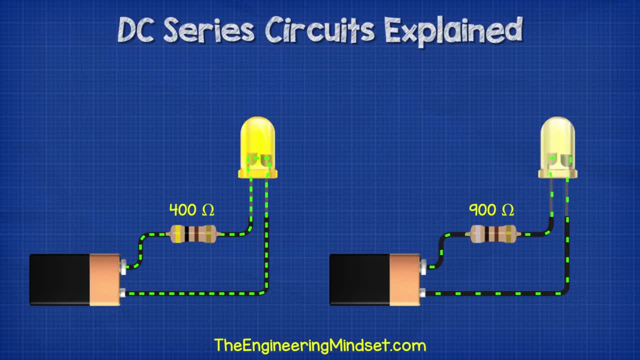 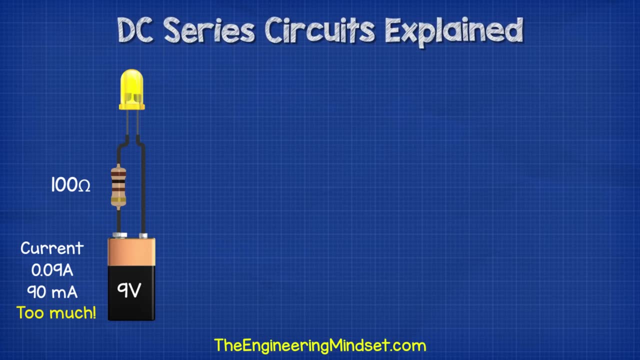 an LED with a resistor into a circuit. The higher the resistance, the dimmer the LED will be. We can also use resistors to protect components in the circuit. If I use a 100 ohm resistor with a 9 volt battery, the current will be around 0.09 amps. 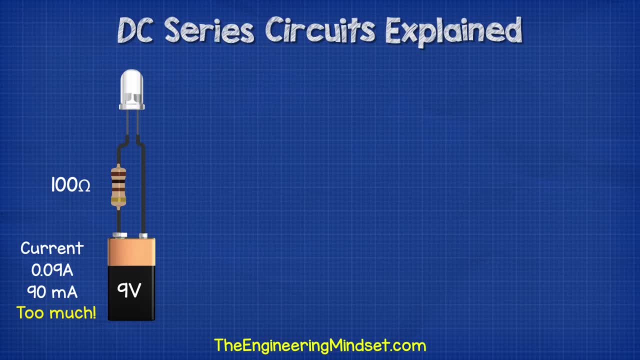 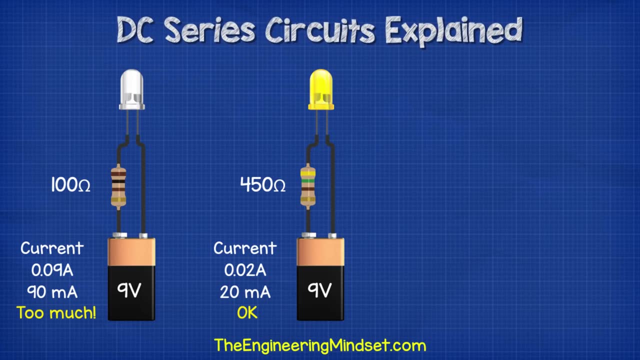 or 90 milliamps and that will be too much and it will blow the LED. If I use a 450 ohm resistor, the current will be around 0.02 amps or 20 milliamps, So the LED should be ok. 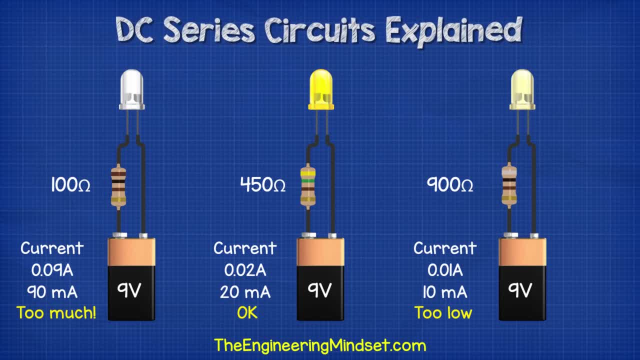 If I use a 900 ohm resistor, the current will be 0.05 ohms and the current will be 0.05 ohms, The current will be 0.01 amps or 10 milliamps and the LED will be very dim then. 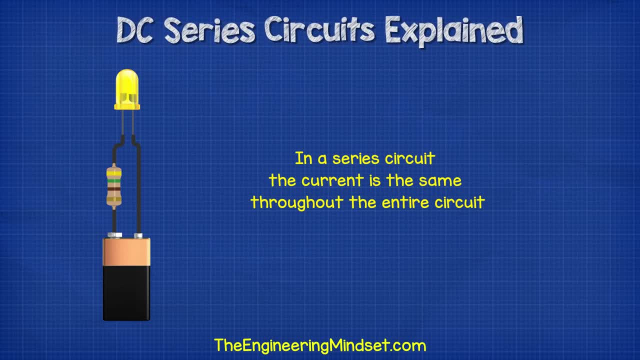 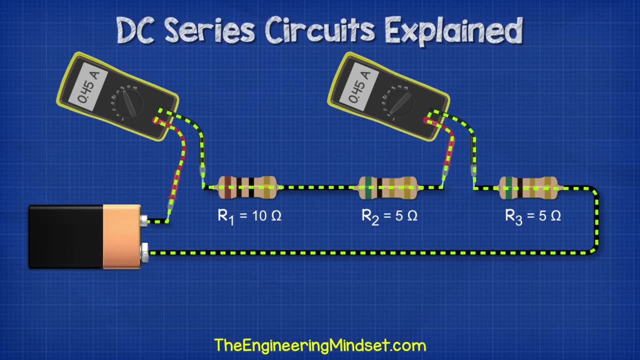 In a series circuit, the current is the same throughout the entire circuit. That's very important. so do remember that If we place the meter here or here, we will get the same reading. That's because there is only one path for the electrons to flow, and they will all move. 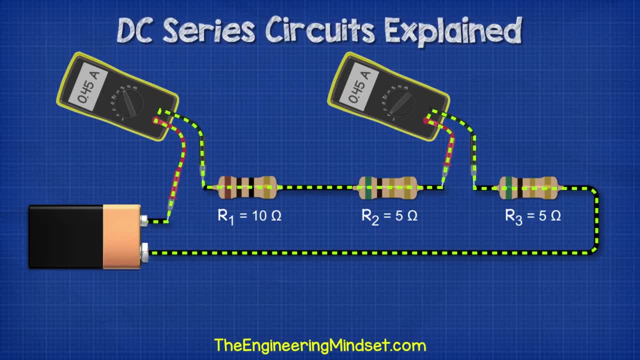 together in the same direction, so the current must be the same. It doesn't matter where we measure or where we place the resistor. even if we swap the order of the resistors, the current will be the same anywhere in a series circuit. 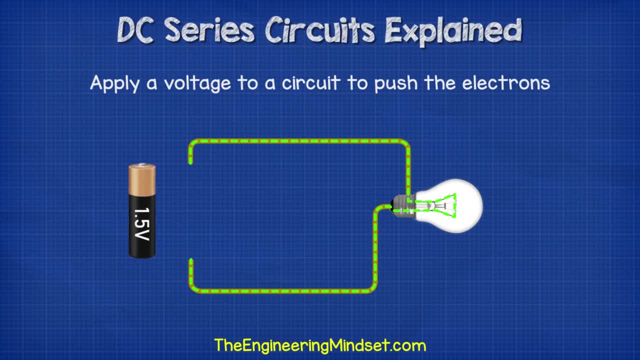 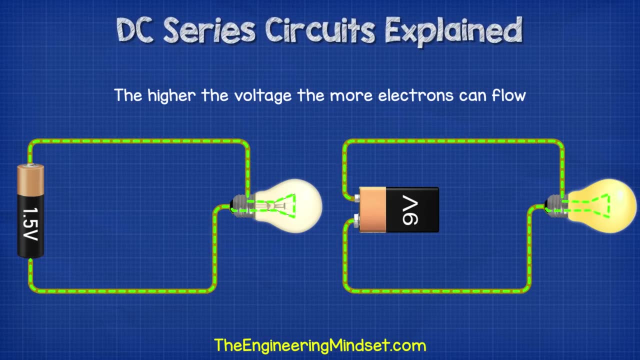 Voltage in series. Remember, voltage is the pushing force of electrons. It's like pressure in a pipe: The higher the pressure, the more water can flow. The higher the voltage, the more electrons can flow. We can see that by varying the voltage to a lamp, as illustrated here. 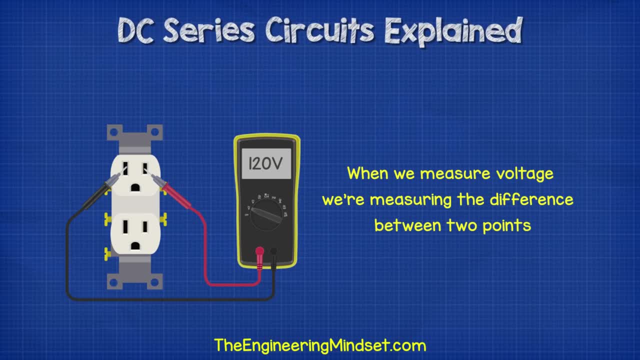 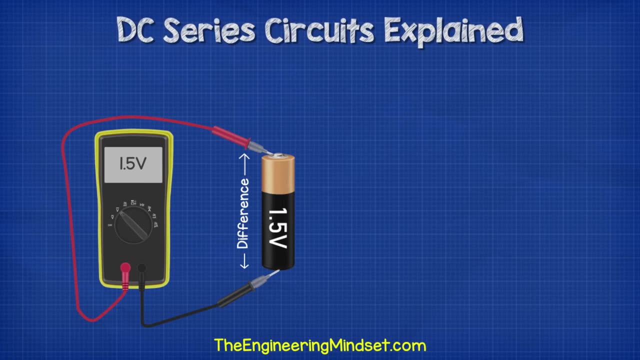 The lamp increases in brightness as the voltage increases. When we measure voltage, we're measuring the difference, or potential difference, between two points. If we read across a one point five volt battery, we get a reading of one point five volts, But if we try to measure the same side, we wouldn't read any voltage. 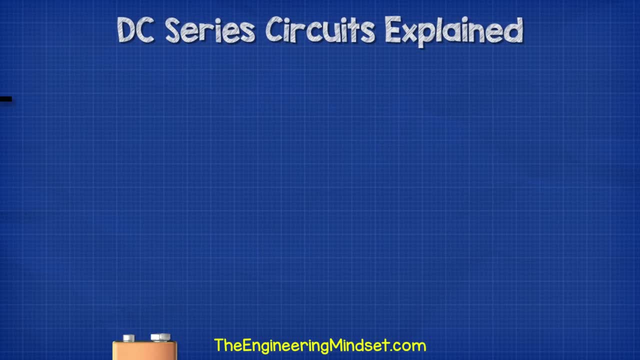 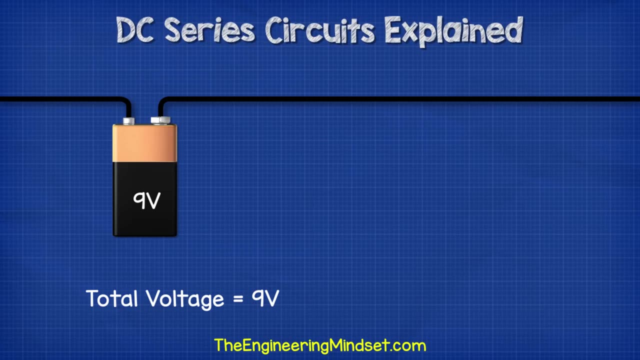 We can only measure the difference between two points. If we place a 9V battery into the circuit, we apply 9V to the circuit. We can increase this by wiring the batteries in series. So if we place two 9V batteries in a circuit in series, then we get 18V. 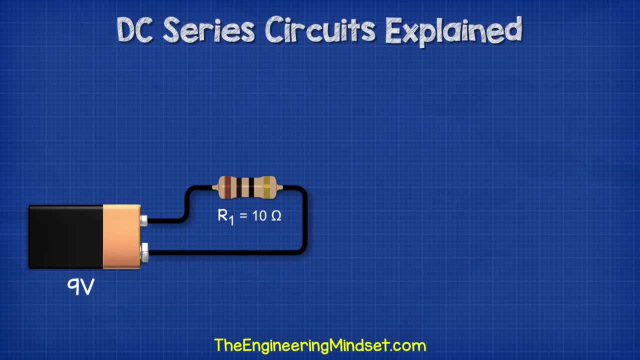 Three 9V batteries will give us 27V. Let's take a 9V battery and add an R1 resistor of 10Ω to the circuit. If we use a multimeter to measure across the resistor, we get a voltage reading of 9V. 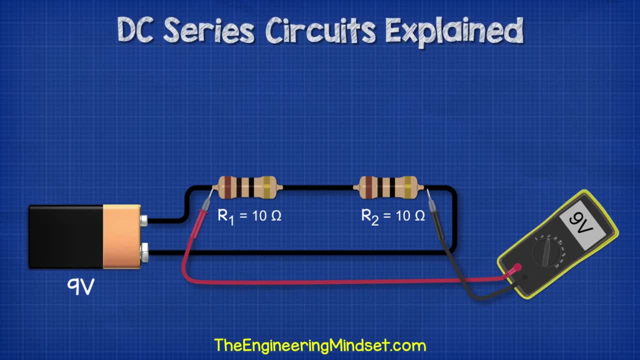 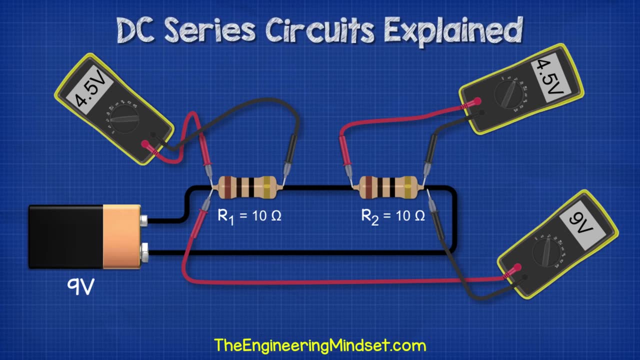 If we add another 10Ω resistor, we get a reading of 9V across the two resistors, But we get a reading of 4.5V if we measure across either of the resistors individually. So the resistors are dividing the voltage. 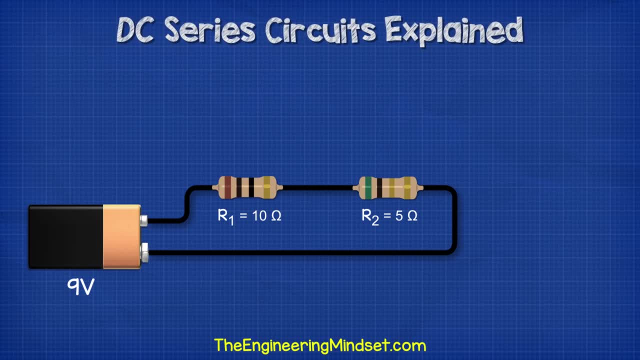 If we replace the R2 resistor with a 5Ω resistor, the total voltage would again be 9V. And that's what we see if we measure across the two resistors. But if we measure across the 10Ω resistor, 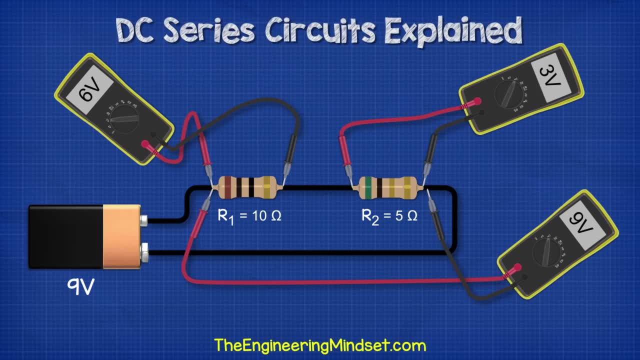 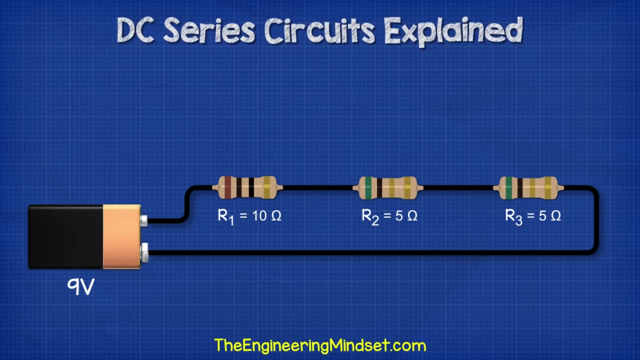 we see a voltage of 6V and if we measure across the 5Ω resistor we see 3V. We'll look at why that is just shortly If we added another resistor- R3, with 5Ω into the circuit. 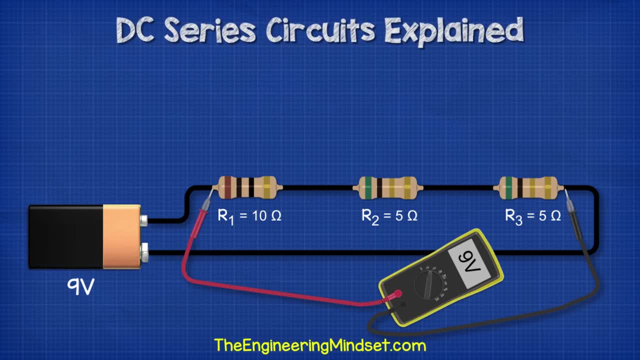 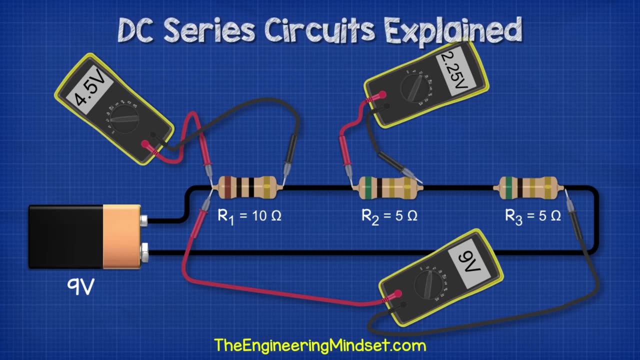 we again get a total voltage drop of 9V across the three resistors. Across the R1 10Ω resistor, we read 4.5V. Across the R2 5Ω resistor, we read 2.25V. 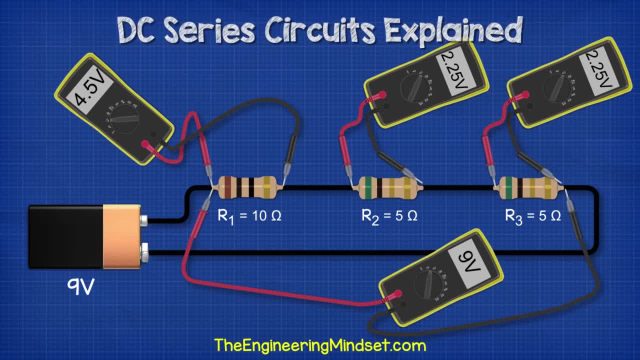 and across the last R3 5Ω resistor we again see 2.25V. We can combine these results and we get a total voltage drop of 9V across the three resistors. We can also use these readings to find the voltage at different parts of the circuit. 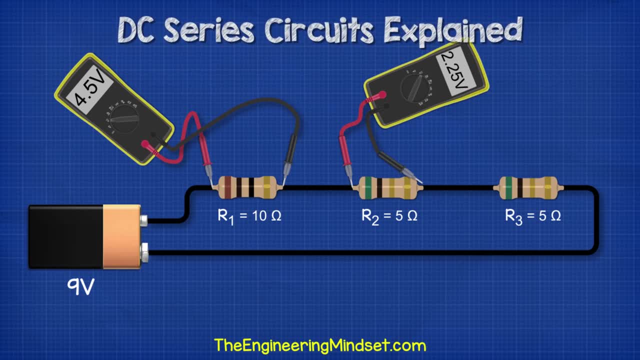 For example, if we measure from the battery across R1, we see 4.5V. If we measure from the battery across R1 and R2, we get 6.75V, because 4.5V plus 2.25V. 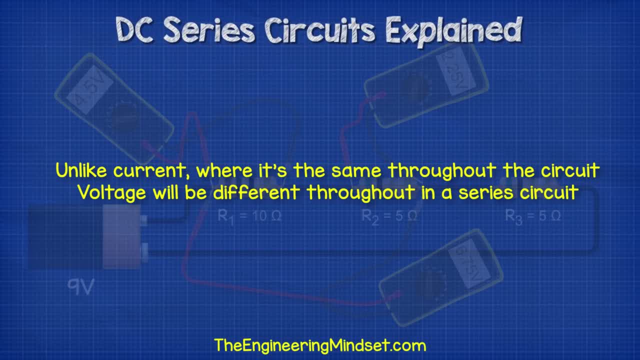 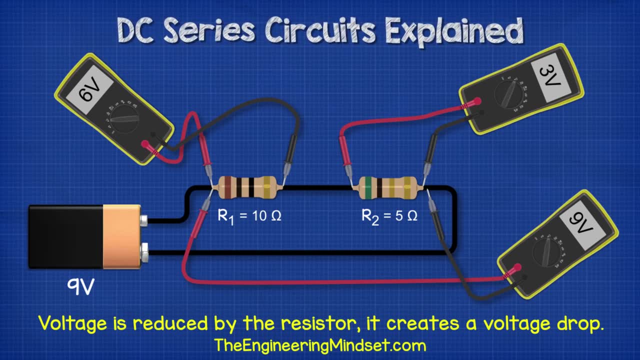 So, unlike current, where it's the same throughout the circuit, the voltage will be different throughout a series circuit. This shows us that the voltage is reduced by each resistor, so the resistor creates a voltage drop. That's the purpose of the resistor. 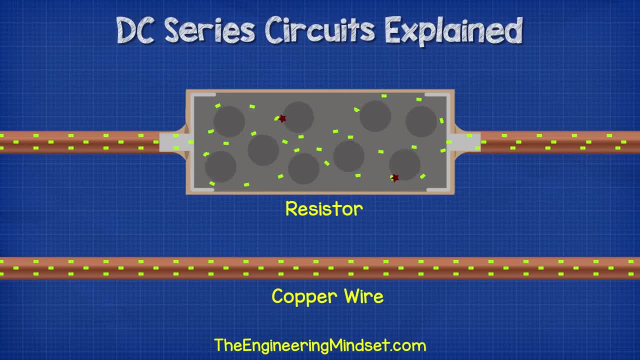 to reduce the voltage or the pressure. What's happening is, the resistor creates a more difficult path for the electrons to flow through and as they flow through, they will collide with other electrons. This collision will convert the energy into heat. The same amount of electrons will enter and exit the resistor. 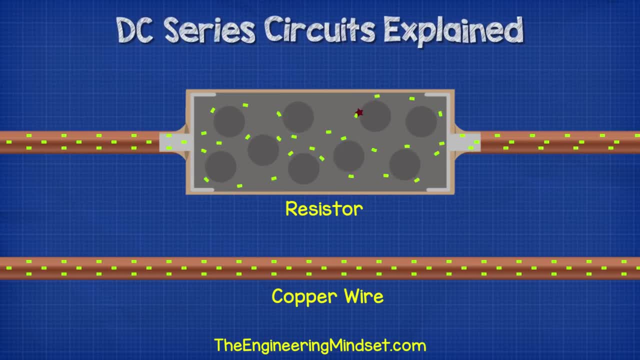 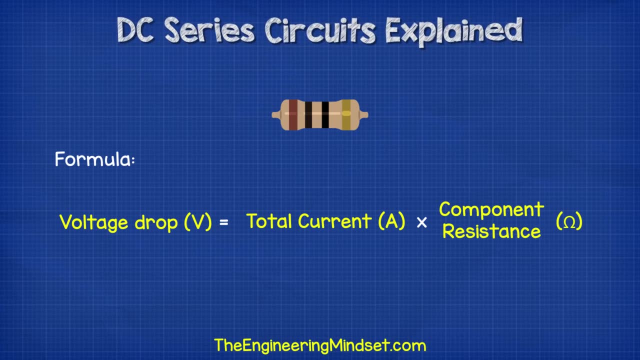 they will just have less energy or pressure as there's been a voltage drop. We can calculate the voltage drop across each resistor individually by multiplying the total current in the circuit by the resistance of each component. Remember, in a series circuit the current is the same anywhere in the circuit. 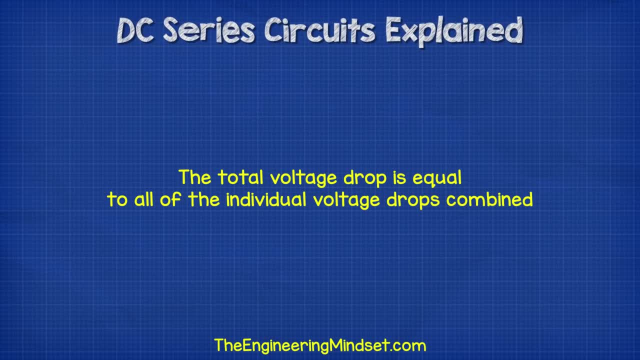 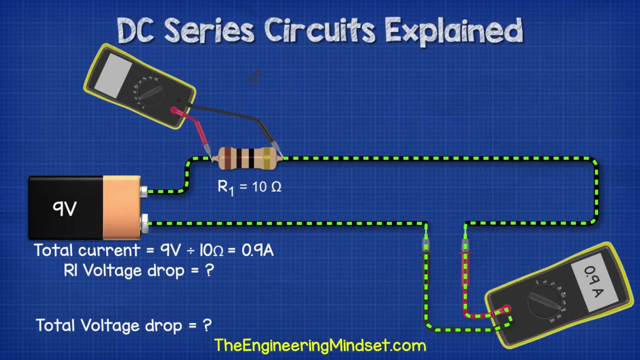 The total voltage drop will be the total of all the individual voltage drops combined. The first circuit there was a 10Ω resistor. by itself The circuit had a current of 0.9A. so 0.9A multiplied by 10Ω equals 9V. 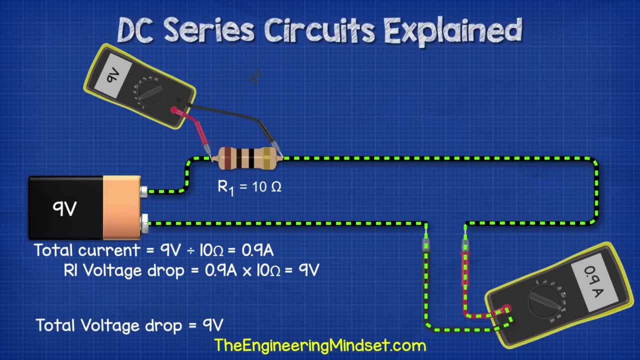 The voltage drop across the resistor is therefore 9V, and that's the same as the voltage source. The second circuit had a 10Ω and a 5Ω resistor together. the 2nd circuit had a 10Ω and a 5Ω resistor together. 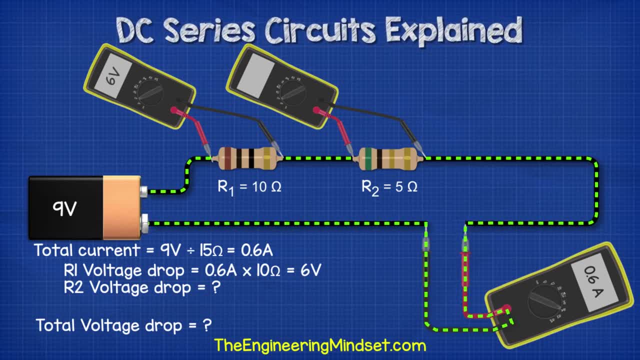 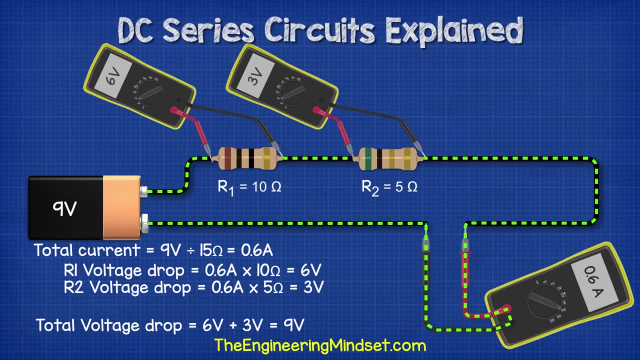 first resistor voltage drop is 0.6 amps multiplied by 10 ohms, which gives us 6 volts. The second resistor was 5 ohms and the current was the same. so 0.6 amps multiplied by 5 ohms equals 3 volts. 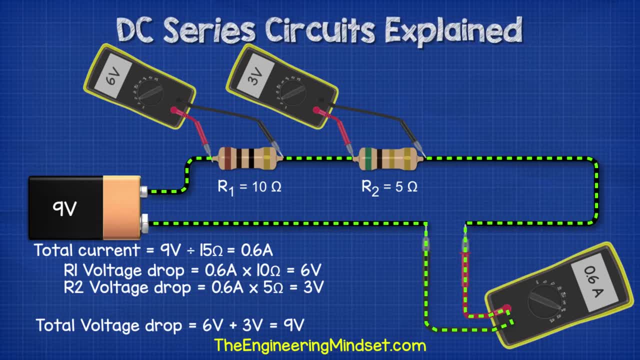 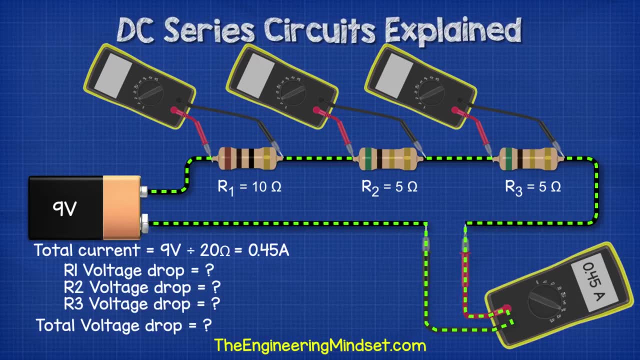 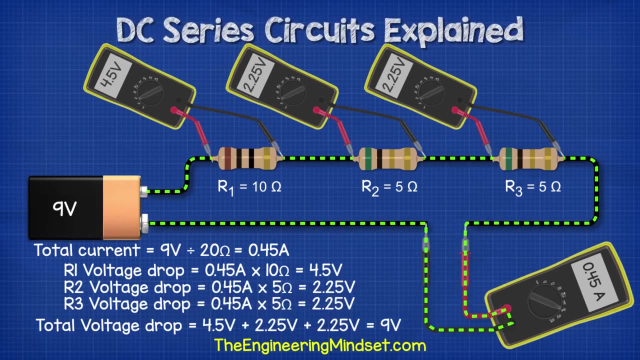 The total voltage drop is therefore 6 volts plus 3 volts, which gives us our 9 volts. The third circuit has a 10 ohm and two 5 ohm resistors. The circuit had a current of 0.45 amps, so R1 is 0.45 amps multiplied by 10 ohms, which gives us 4.5 volts. R2 and R3 will be 0.45. 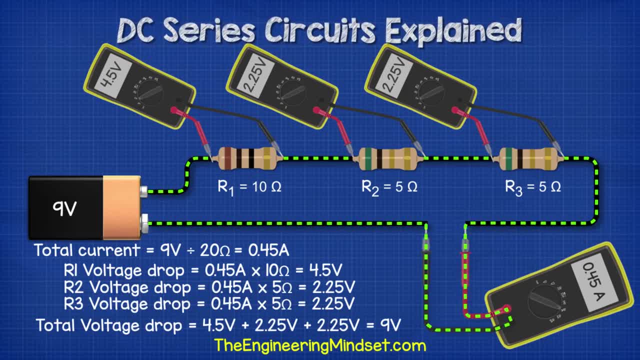 amps multiplied by 5 ohms, which gives us 2.25 volts on each, The total voltage drop is therefore 9 volts, which is 4.5 plus 2.25 plus 2.25.. Power consumption in series circuits. How do we measure? 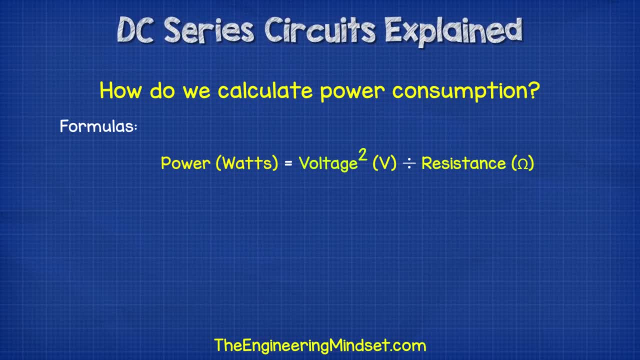 power consumption of the circuit. Well, we can use the following equations: We can either use power consumption in series circuits, or we can use power consumption in series circuits. Power, which is watts, equals voltage squared divided by resistance. or we can use power equals voltage multiplied by current. You might be wondering how can a resistor consume power? 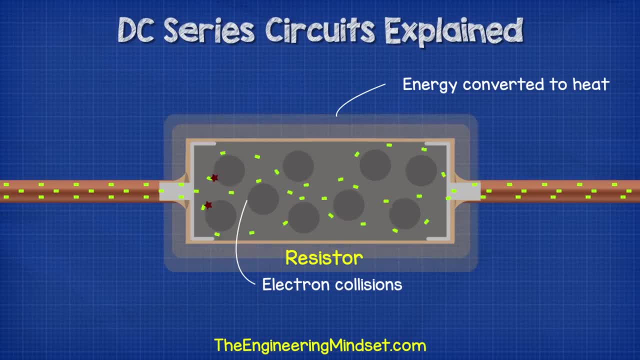 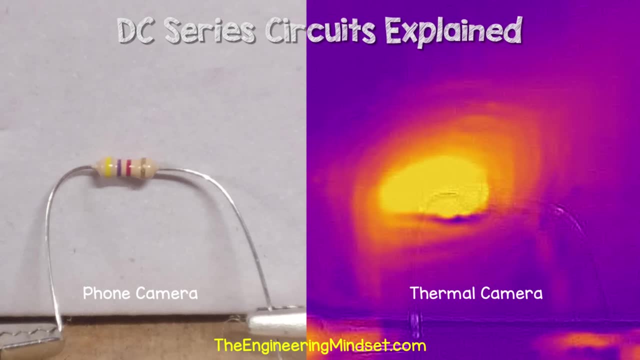 Well, as the resistor is creating a voltage drop, the electrons are losing some energy. Where is this energy going? Well, the electrical energy is being converted into heat, and if we look at some resistors under a thermal imaging camera, we can see the heat is being. 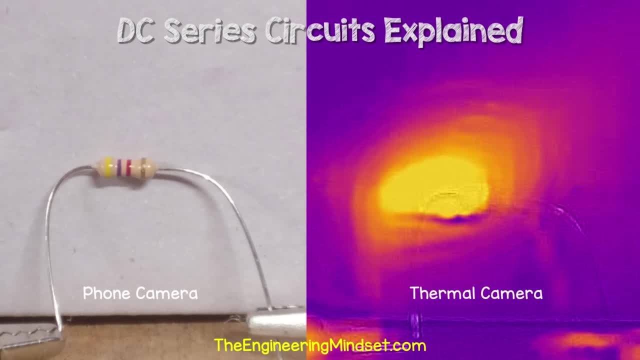 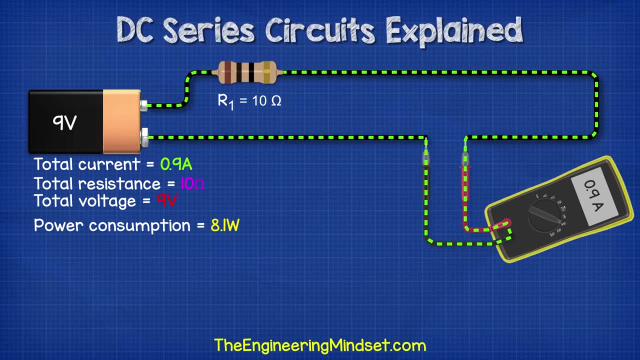 generated, So the power consumption is actually the heat being dissipated from the circuit. So in this circuit the resistance is 10 ohms, the battery is providing 9 volts, the current is 0.9 amps and the circuit consumes 8.1 watts of power. How do we calculate that, Using method 1, 9 volts squared? 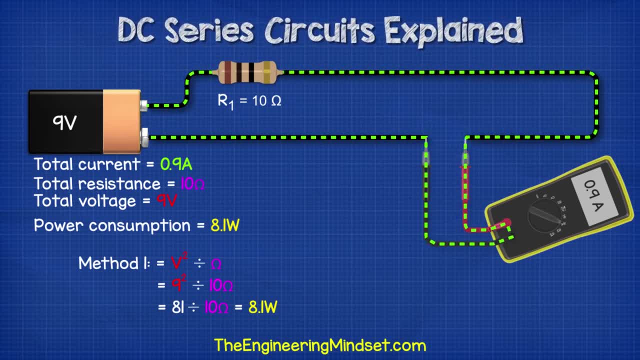 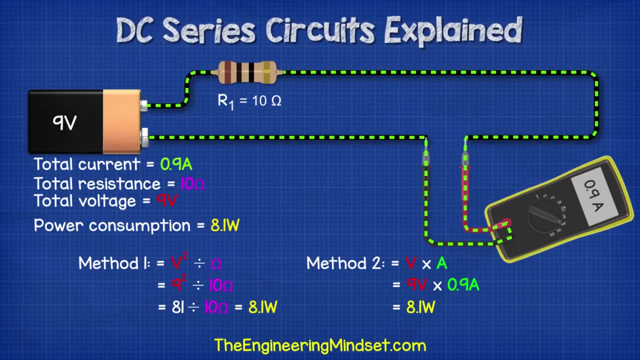 or 9 multiplied by 9 is 81. divided by 10 ohms is 8.1 watts. Alternatively, 9 volts multiplied by 0.9 amps equals 8.1 watts. In the circuit, with the 10 ohm and the 5 ohm resistor, the total resistance. 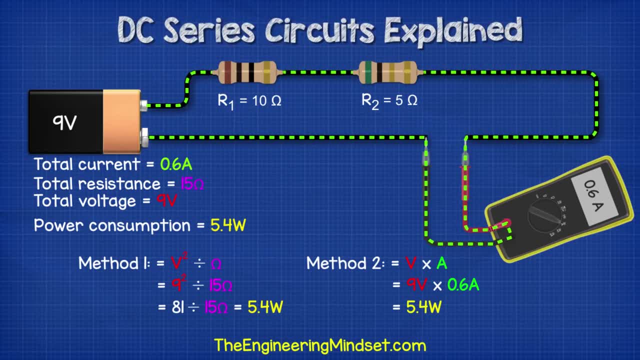 was 15 ohms, So the resistance is 10 ohms. divided by 10 ohms, which is 8.1 watts, So the resistance is 10 ohms and the current was 0.6 amps, So 9 volts squared is 81. divided by 15 ohms is 5.4 watts.